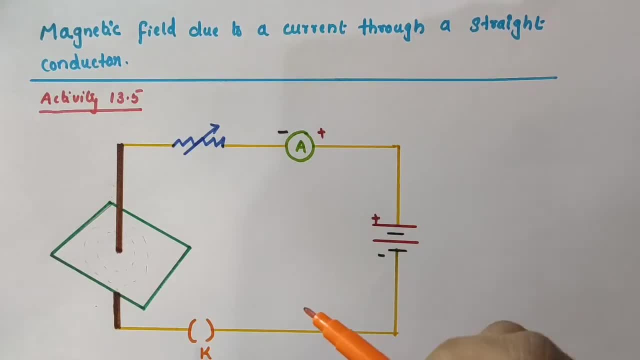 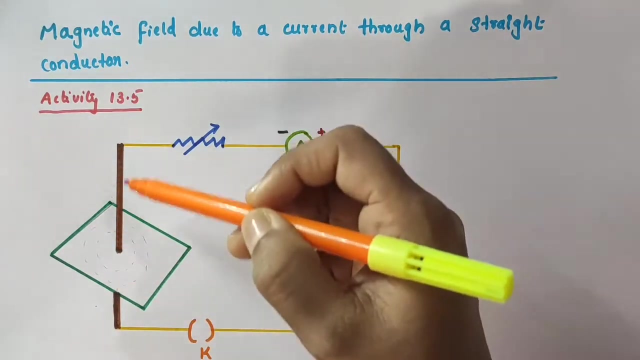 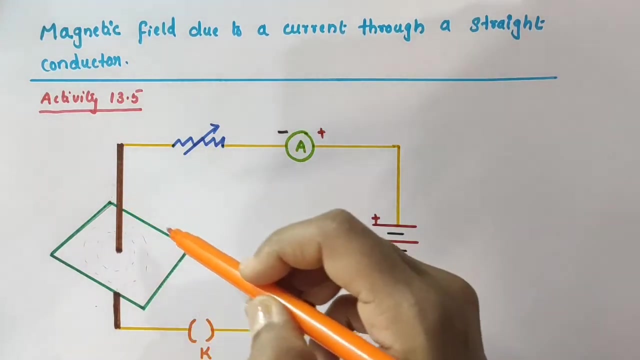 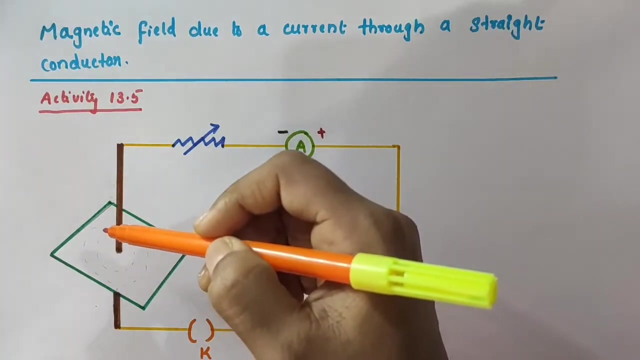 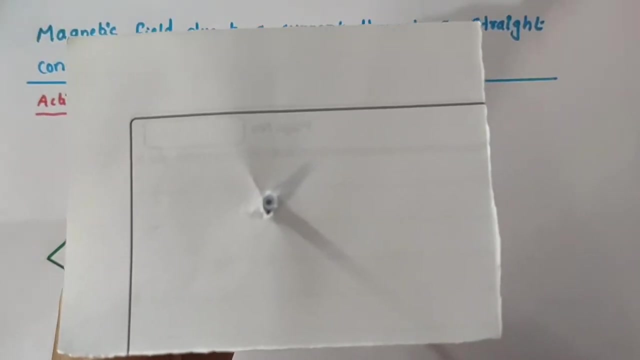 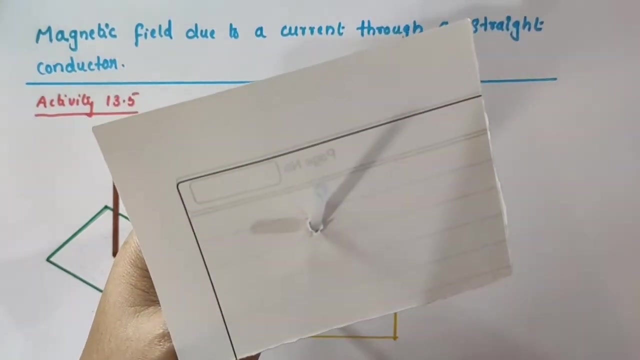 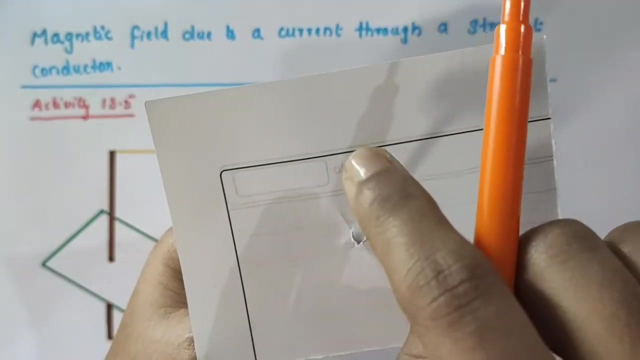 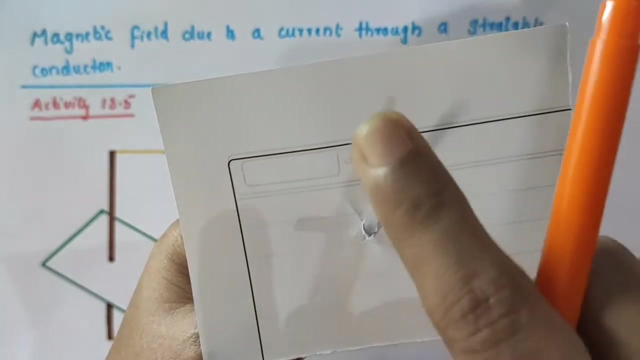 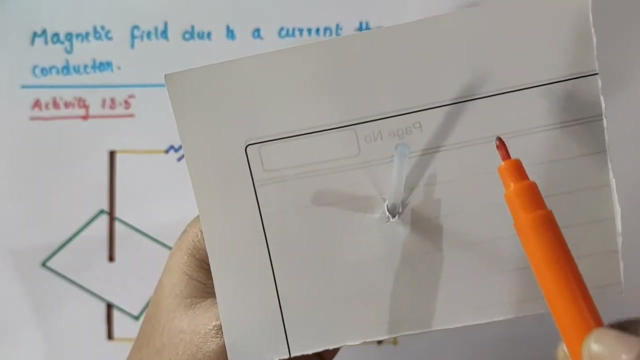 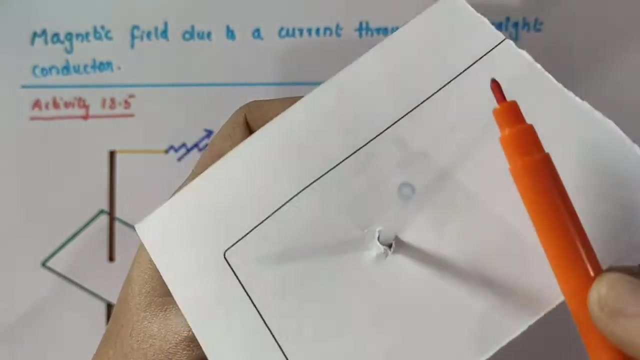 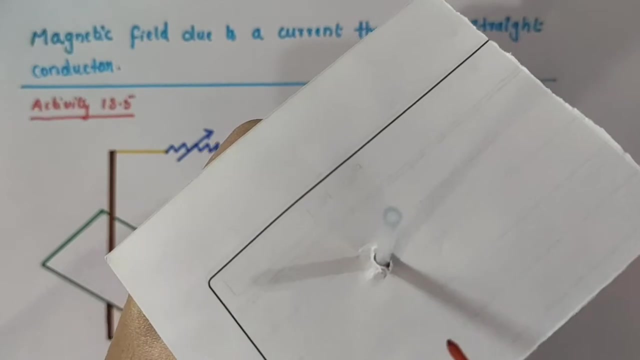 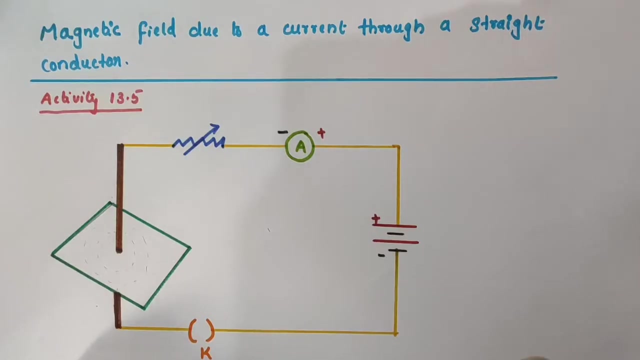 Hello everyone. In this video, we are going to discuss about the pattern of the magnetic field around a straight conductor carrying current. First, let us discuss about the activity 13.5. For this activity, we want to take a battery of 12V, a plug key, a long straight thick copper wire, this brown colored one is the copper wire, then a rheostat or a variable resistance, then an ammeter of range 0 to 5 ampere and a rectangular cardboard. This green colored one is a rectangular cardboard. And we want to make a connection as shown here. Here, this thick copper wire is actually inserted through the center of this rectangular cardboard and this copper wire is placed in such a way that it is normal to the plane of the rectangular cardboard. That is like this. I hope you can see this. Okay, you just imagine. I don't know whether you are able to see this. Okay, I hope you can see this. You just imagine this as the rectangular cardboard and this one as the thick copper wire. So, this copper wire is inserted through the center of this rectangular cardboard and the copper wire is inserted through the center of this rectangular cardboard and it is actually you can see that this copper wire is perpendicular to the plane of this cardboard. Okay, it must be fixed here. Okay, you can see here. This one is a straight one like this and the plane of that paper is here. So, cardboard is like this and the copper wire is like this. The copper wire is perpendicular to the plane of the cardboard. So, this copper wire is inserted here. It should not slide up or down. Okay, then we want to sprinkle some iron filings uniformly on the cardboard. When the key is closed, a current flows through the circuit from the positive terminal to the negative terminal. So, a current flows through this circuit like this from the positive terminal to the negative terminal and using the current flows through this copper wire too. 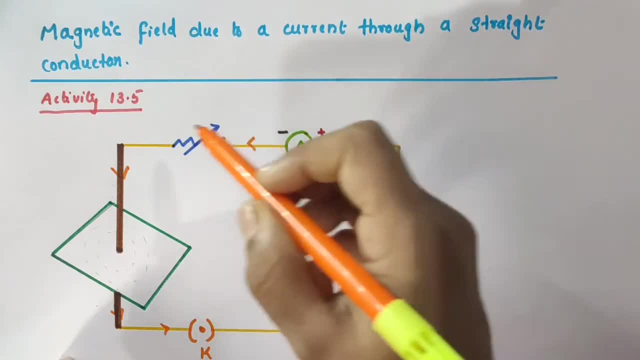 And using the amine. We can determine the value of that current flowing through the circuit. 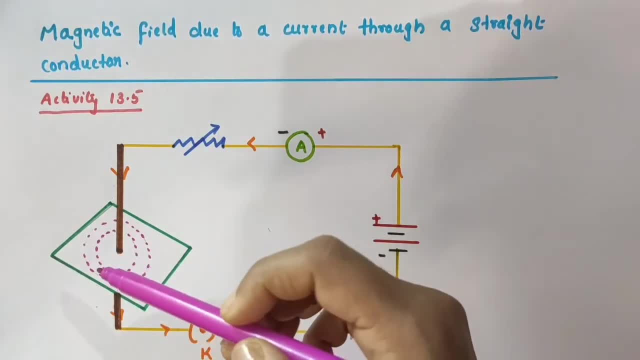 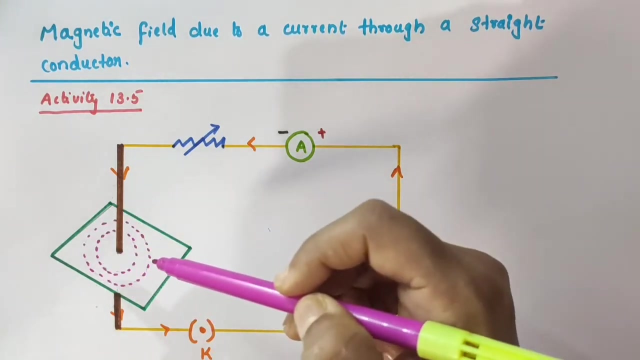 When we gently tap the cardboard a few times, we would observe that the iron filings align themselves showing a pattern of concentric circles around the copper wire. You just consider these pink colored dotted ones as the iron filings. So, when we gently tap the cardboard a few times, the key is closed, current is flowing through this copper wire. 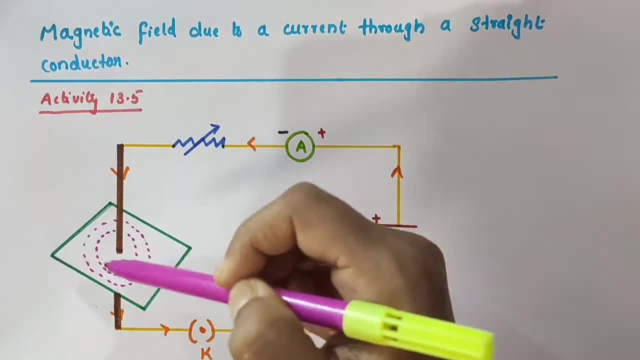 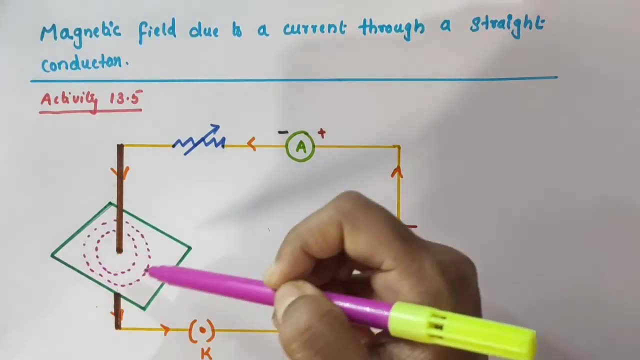 aboみ which is a kind of coffee神 which is a呼声 that, if you analyze cartoons or books, you would have heard that in our country, they say that strong winds contaminate the surface with abundant DNA buying in the form of plasma produced by brass. We can homeland basically meters. Image image Women having a baby just taking the sperm from the body smaller forms of magnetic field is trained as движable while making a circle around the paper swab konkak Oliver 1946 975 the pattern of constantly circles indicate the field alliance of a magnetic field around the street the call conducting wire. Positive way of meget うир übergeoma The 보는 is not including the magnetic field around the current curing straight wire become larger and larger. YES THAT IS WHAT WE ALSA FEEL. 이вонқ as we move away from it. quindi Why are we getting it? So, we obtain the pattern of the magnetic field. In Voilà see what it looks like 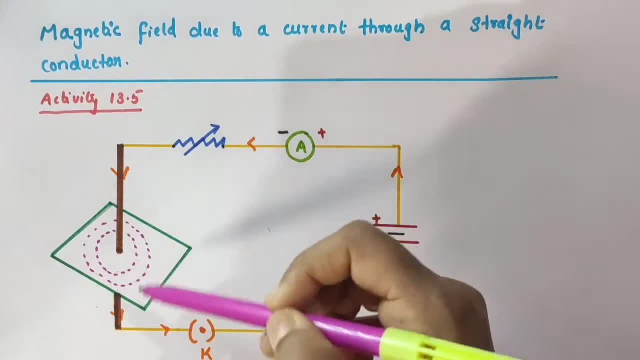 field around a straight conductor carrying current as concentric circles magnetic field is a vector conditino so it has a direction it has both magnitude and direction how can the direction of the magnetic field be found for example if you want to determine the direction of magnetic field at this point P okay I'm considering a point P here then we just want to place a compass needle at this point P okay then the direction of the North pole of that compass needle will give the direction of the magnet field lines 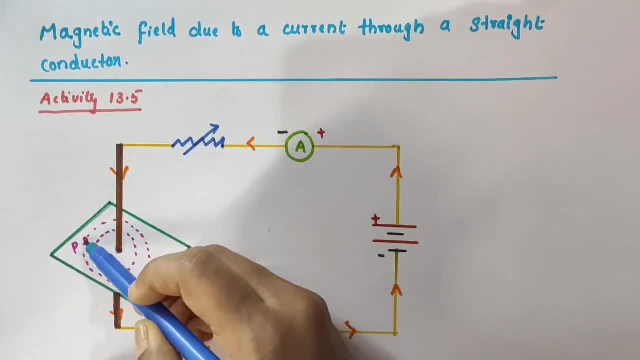 produced by the electric current through the straight wire at this point P so I'm just marking the direction of magnetic field lines like this okay I am just marking the direction of magnetic field lines like this that is in the clockwise 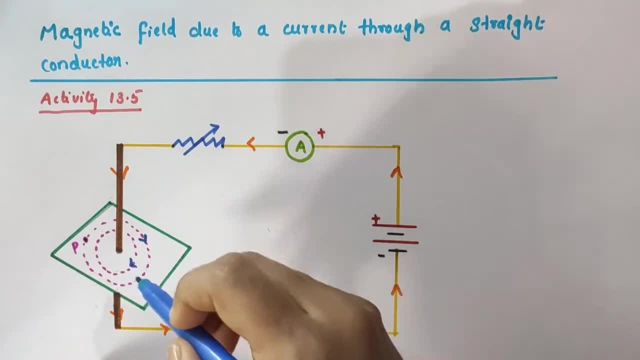 directions alright why did I mark like this that is the My anti-feed lines are moving like this. That is in the clockwise direction. Why did I mark like this? Even without using a compass. 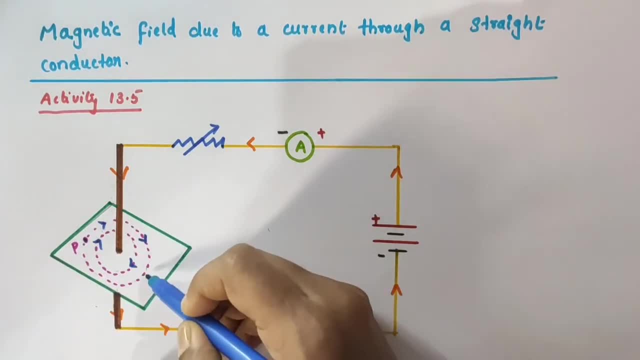 Why did I put the arrow like this? Why didn't I put an arrow like this? That is from here to here in the anti-clockwise direction. 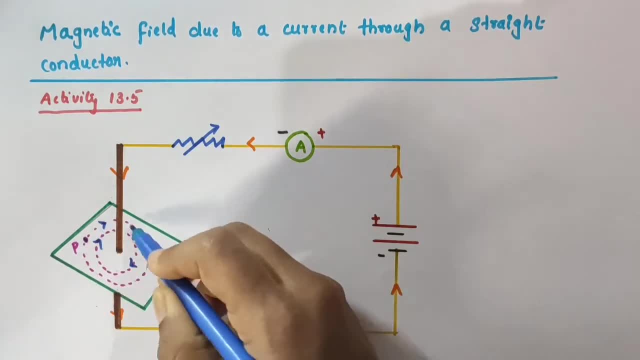 Okay, I marked the arrows in the clockwise direction. No, I didn't mark the arrows in the anti-clockwise direction. 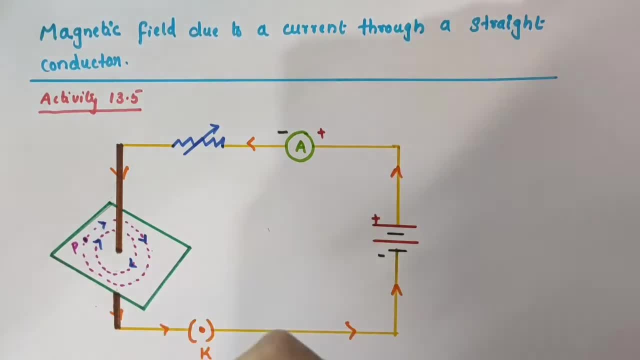 Why? This can easily be determined by using right hand thumb rule which we will discuss in the next video. 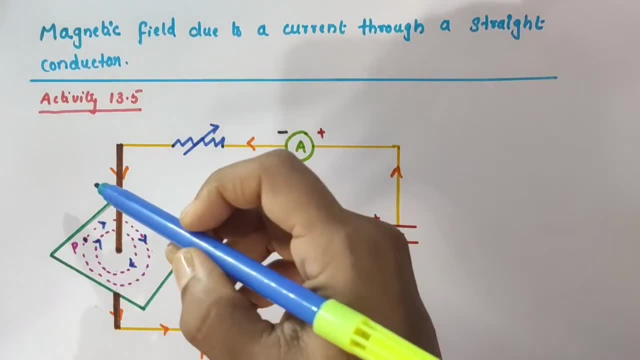 Okay, now see the direction of correction. When through the straight copper wire, when it is reversed, the direction of magnetic feed lines also get reversed. 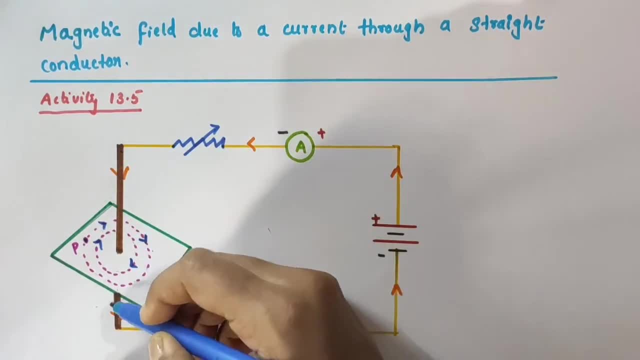 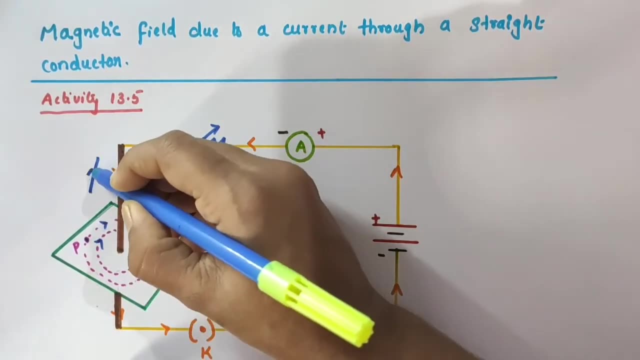 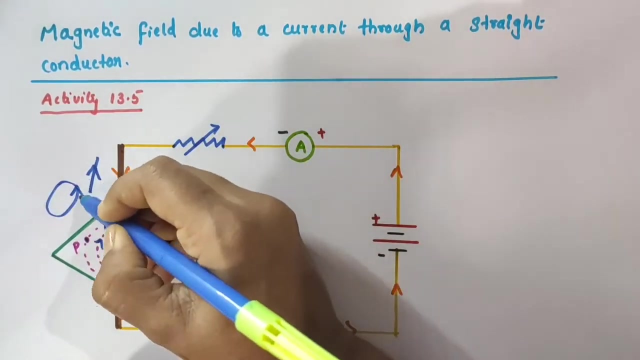 This time, the direction of current from here to here. Okay, and the magnetic feed lines are in the clockwise direction. But when this direction is reversed, that is when the current is going in this direction, flowing in this direction through the copper wire, the direction of magnetic feed lines will be like this. That is in the anti-clockwise direction. Alright, now. 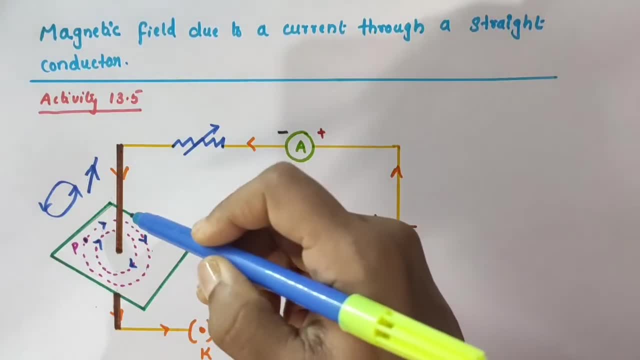 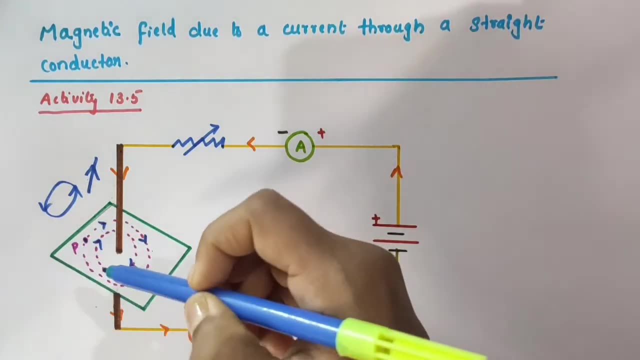 When we vary the current in the wire, in the copper wire, like 1 ampere, 2 ampere, 2.5 ampere, 3 ampere like that, the deflection in the compass needle kept near the wire also changes. In fact, if the current is increased, the deflection also increases. 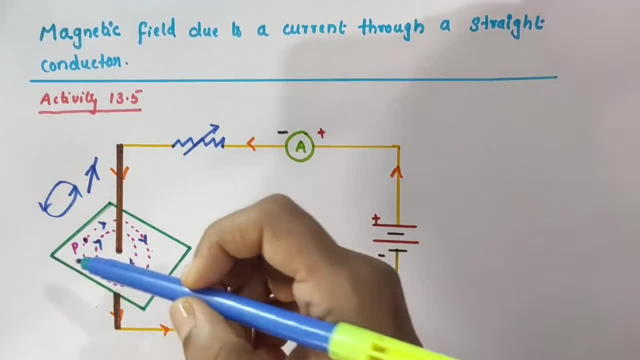 That is, the magnitude of the magnetic field produced at a given point increases as the current through the wire increases. 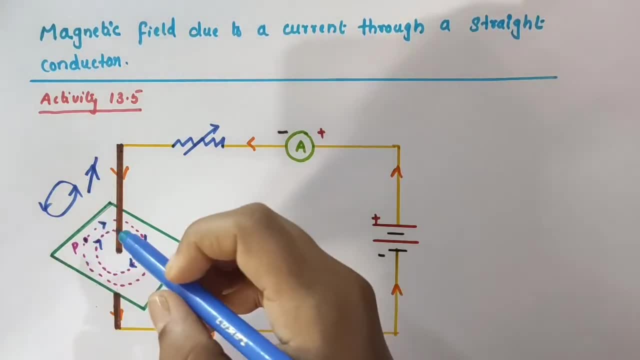 Now, when the compass is moved from the copper wire, and placed at a farther point from the conducting wire, say at a point Q, somewhere here, and current through the copper wire remains the same, then the deflection in the needle decreases. 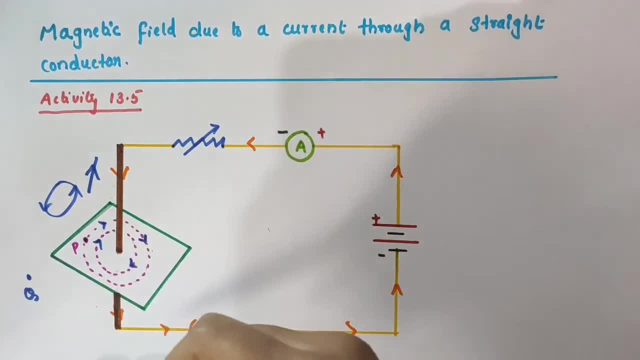 When we are keeping that compass needle somewhere here, the deflection in the needle decreases. 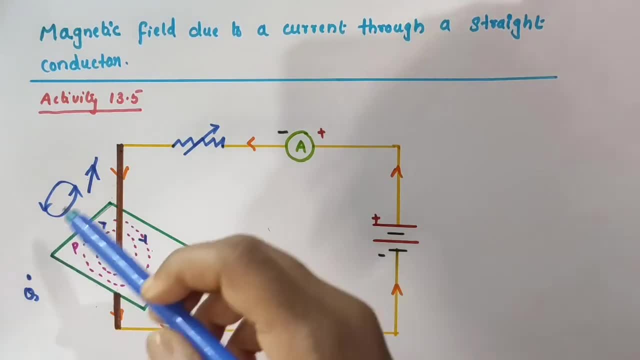 That is, the magnetic field produced at a given current in the conductor decreases as the distance from it increases. Yes.